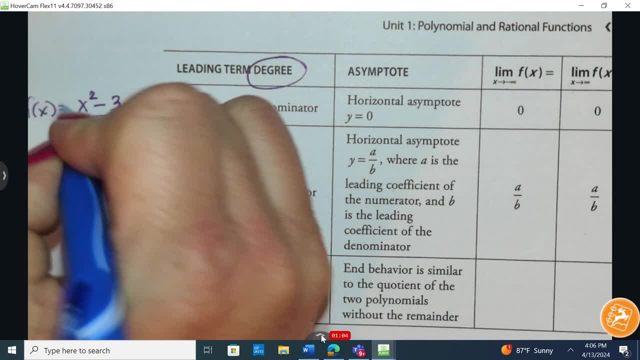 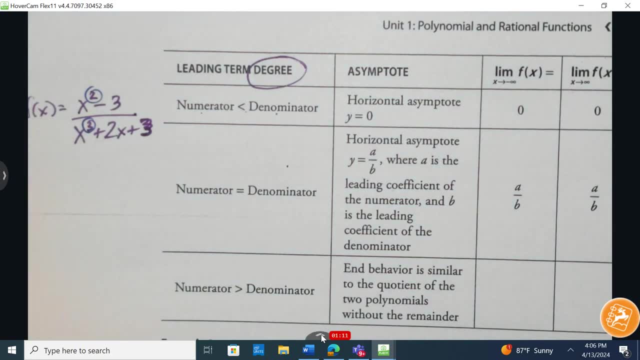 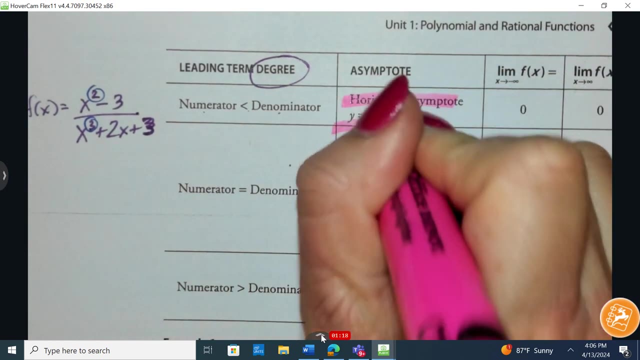 And so if we concentrate on the degree in the numerator and in the denominator, we can see the degree of the numerator is less than the degree of the denominator. Well, what happens when that's the case? When that's the case, we have a horizontal asymptote of y equals zero. 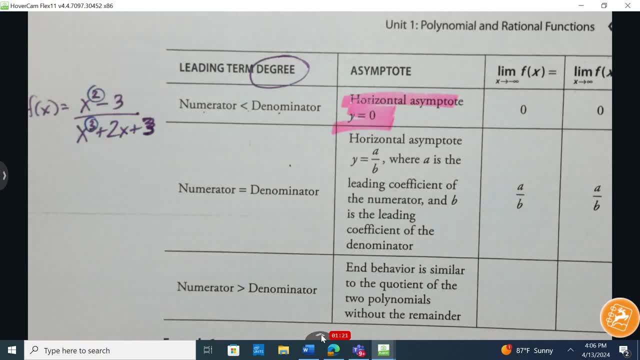 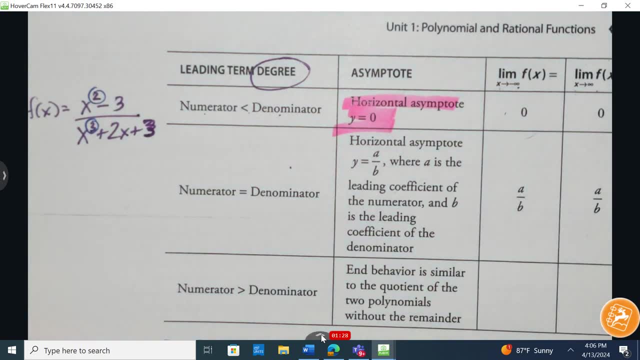 A horizontal asymptote of y equals zero, And how it impacts the end behavior is: as you go to the far left it approaches zero, And as you go to the far right it also approaches zero. So let me just make up an example. 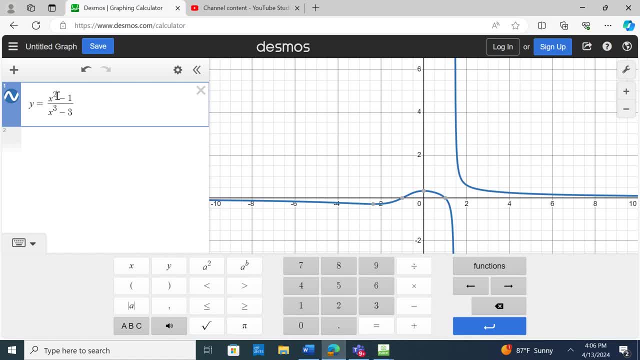 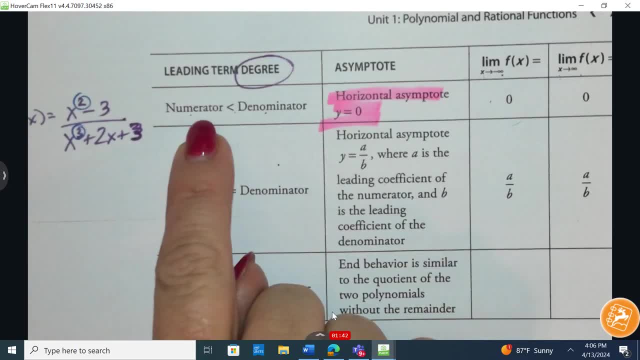 Let me go here to so. I gave us an example where we had a degree of two in the numerator and a degree of three in the denominator, And that's all we're looking for We have. the degree in the numerator is less than the degree in the denominator. 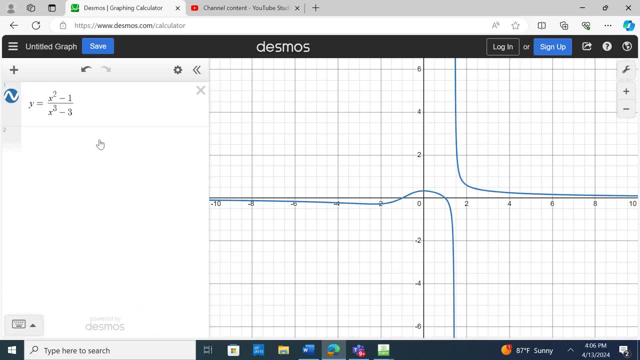 And in that case, if we come back to this, we can see we do have, we do have right here, along this line of the x axis. along this line of the x axis, or y equals zero. If I do that, y equals zero. 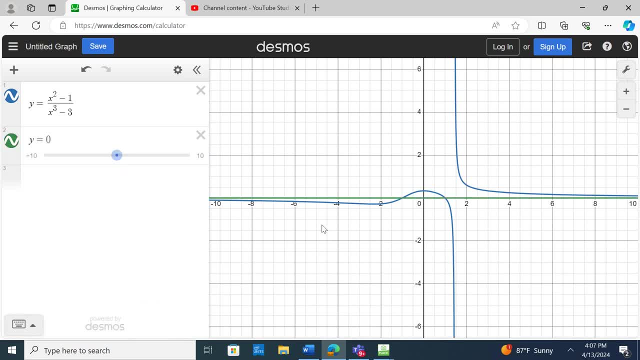 So we have a degree of two in the numerator. We can see that that is going to be, that is going to be our horizontal axis. So on the far left and on the far right we can see it approaches y, equals zero to the far left. 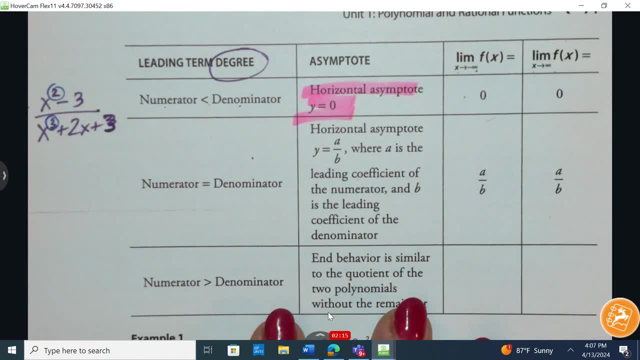 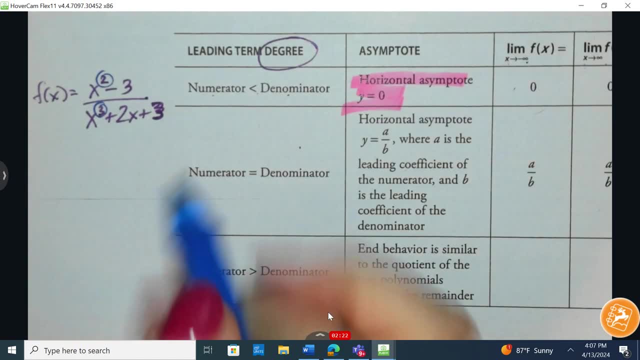 and it approaches y equals zero to the far right. Will that always be the case? It will, And so that's this first rule that we just discussed. Now, what happens when they're equal? What are they talking about being equal? They're talking about the degree. 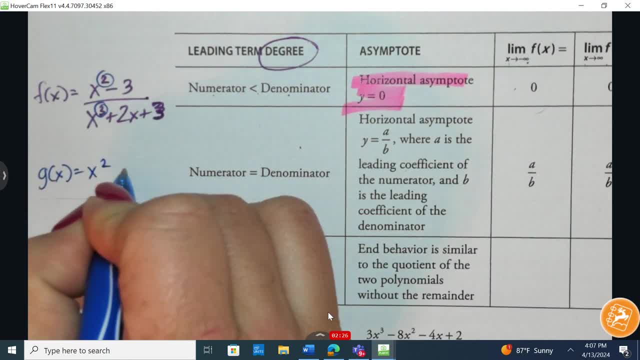 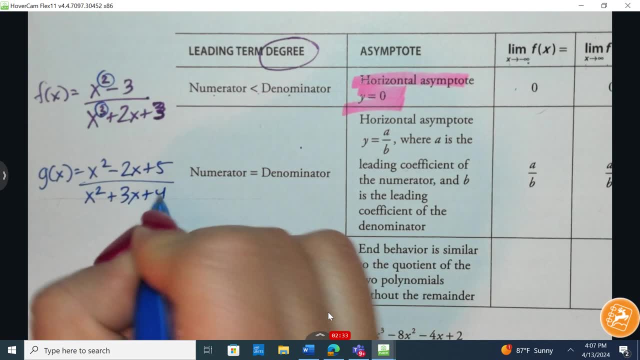 So I can come up with any example here. Let's say x squared minus two, Two x plus five and x squared plus three, x plus four, Completely making those things up. I'm going to come back over here. Let's save ourselves some time. 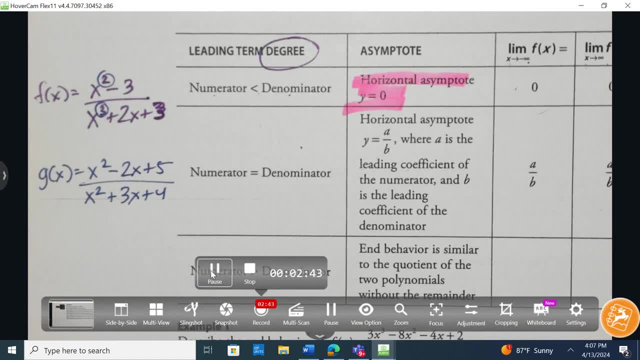 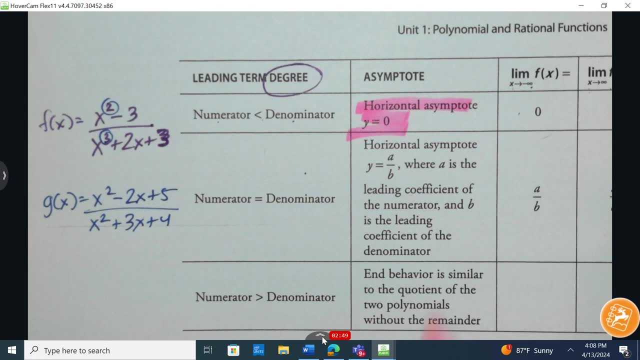 Sorry, let's save ourselves some time. Press play. So if this is the case- and we're going to look in Desmos in just a second- If this is the case, what it says is that we are going to have another horizontal asymptote. 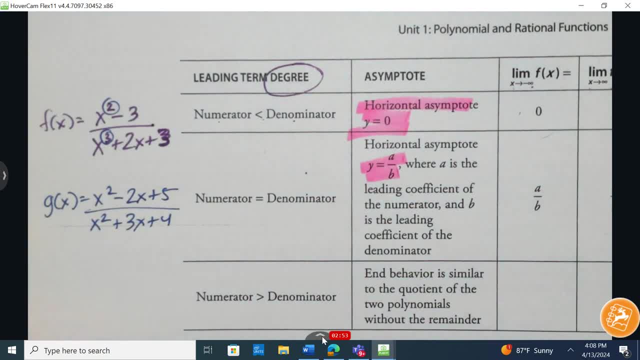 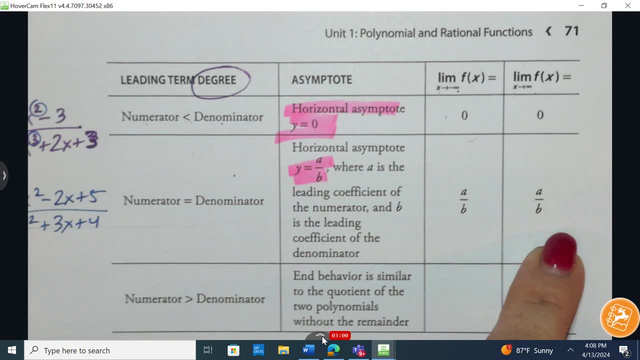 and that's determined by taking the leading coefficient of the numerator and dividing it by the denominator. And the end behavior is: if we go off to the far left it approaches that value And if it goes off to the far right it approaches it. 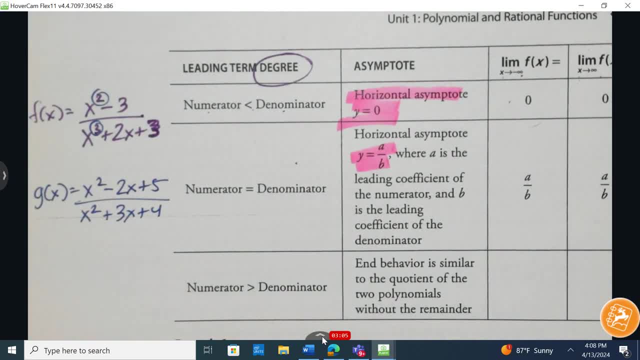 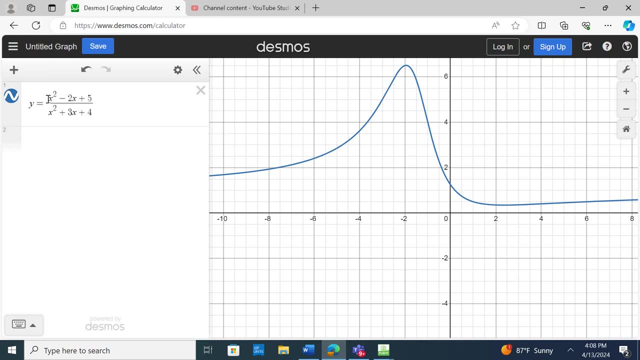 So I plug this particular oops, just a second here. Just dropped the cap on my hollywood calculator. I plug this particular example in. Let's go look at it. And now I can see: the leading coefficient of the numerator and the denominator is one over one. 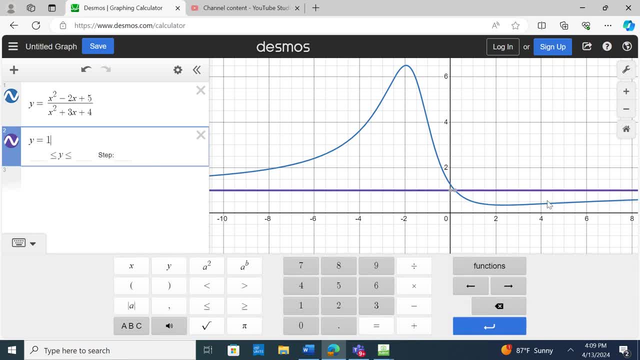 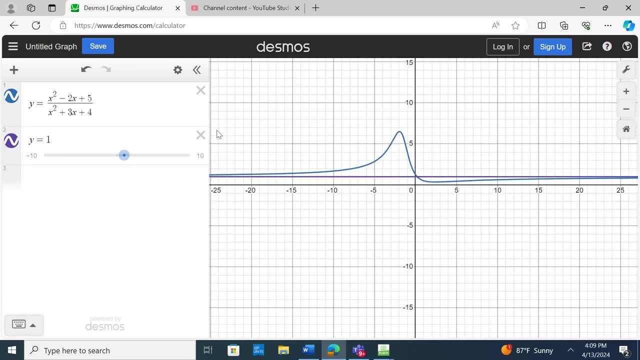 So if I write y equals one, we can see that as I go off to the far left it's approaching that line. as I go off to the far right, especially if I zoom out here, You can see if you go off to the far right and far left. 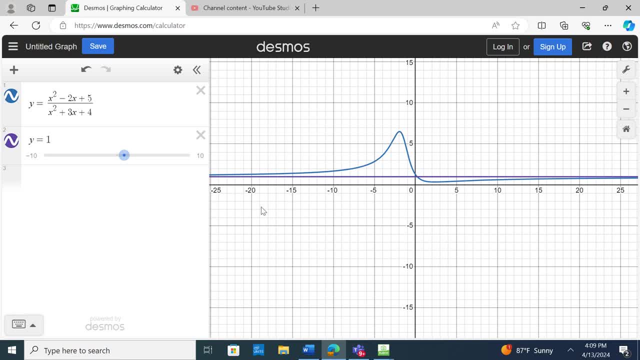 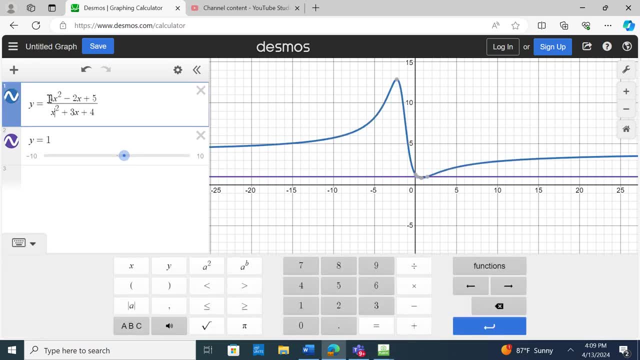 that it is approaching that horizontal, that horizontal asymptote. Now let's just change this up so we can see here, If I just change this up and make this a four and let's make this a seven, well, now I need to change that. 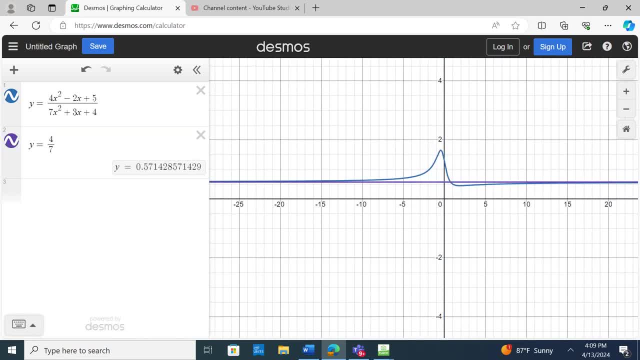 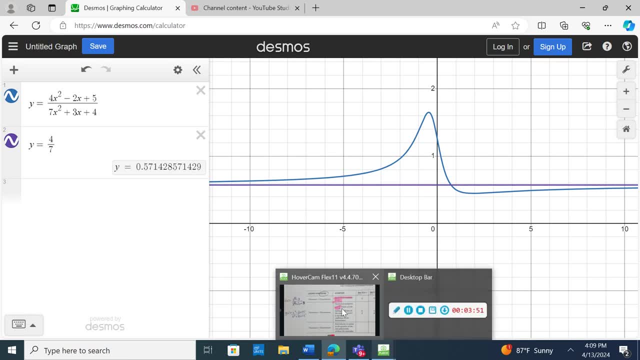 So now this will be four divided by seven, And if you want to zoom in here, you can see as it approaches the far left and the far right. it's going to be the value four sevenths that it's approaching. Let's go to the next one. 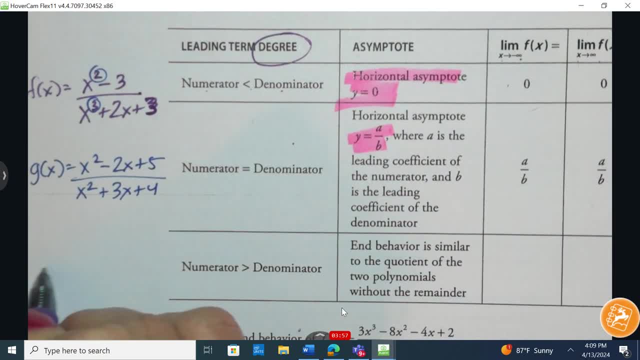 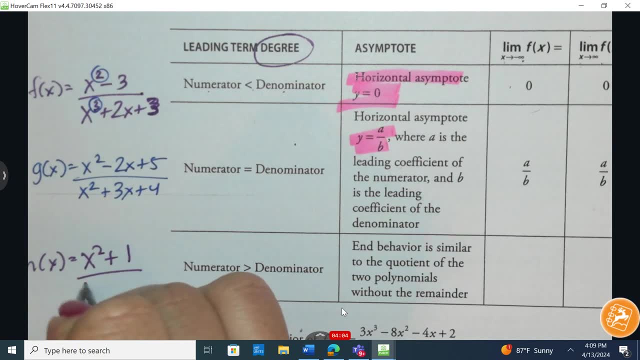 Let's now show an example where the numerator is greater than the denominator. So let's go: h of x is equal to numerator is greater than denominator, So x squared plus one, and this is going to be x minus two. So the end behavior is similar to the quotient of the two polynomials without a remainder. 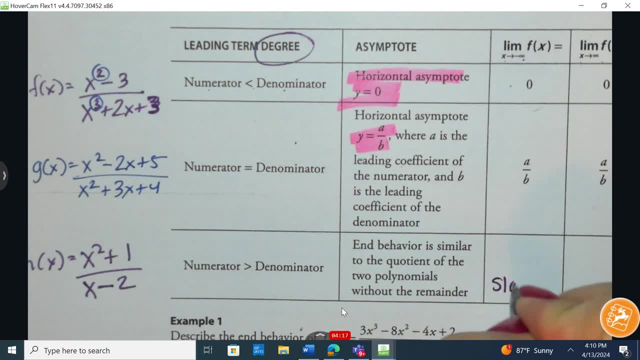 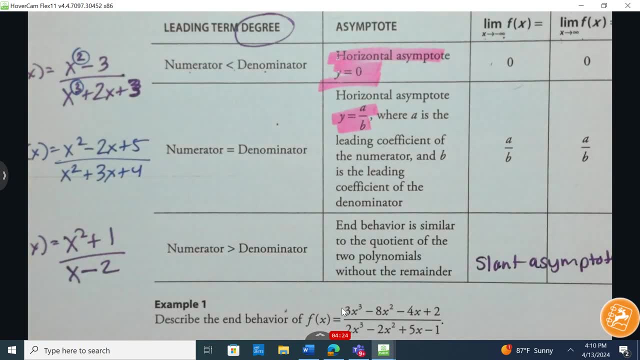 And what that means here is that we have a slant asymptote. You can write that down, slant asymptote. So you're going to do polynomial along division. You're not going to worry about what the remainder is when you do it. 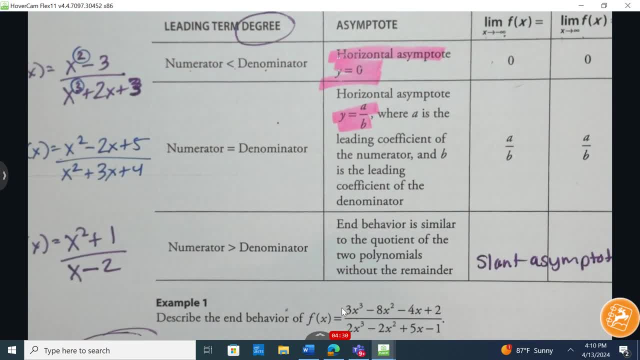 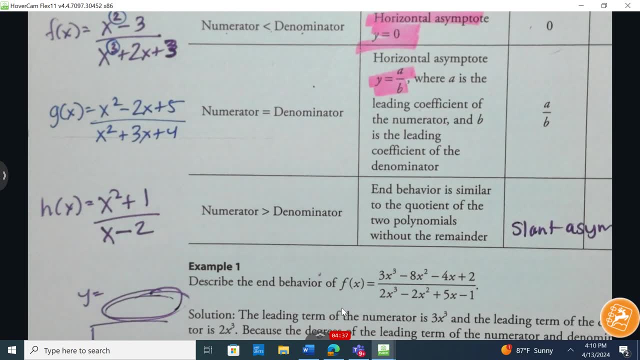 What you have on top. So when we do long division and we divide what we have on top, we're going to write: y equals whatever is remaining and that will be the asymptote, That will be the slant asymptote. So let's take a look and just see what this would have. 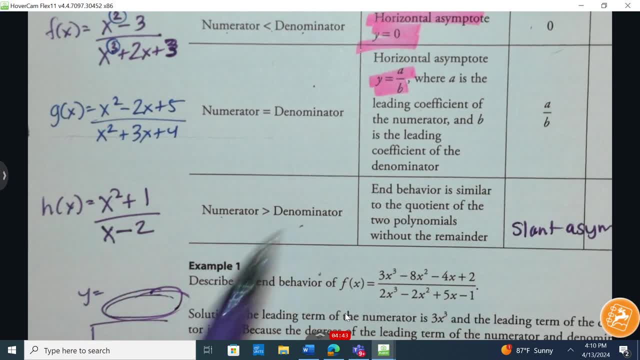 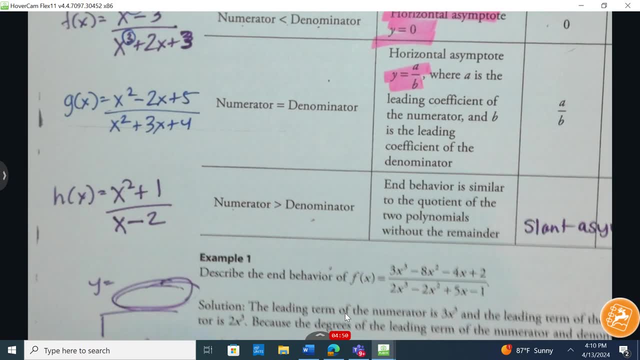 So here we have a two on top, a one on the bottom, So the numerator is greater than the denominator. Okay, so for that situation I need to put the numerator in here, But notice how there's a missing term in the middle. 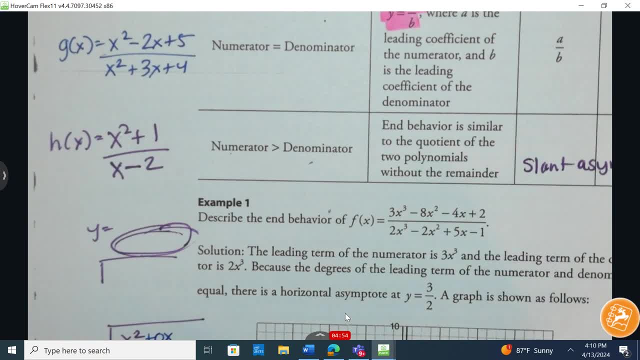 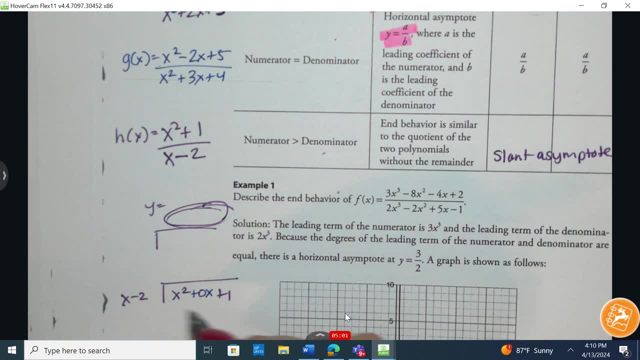 So that needs to be plus zero, x plus one. That missing value needs to be accounted for. On the outside is x minus two. Now I'm going to do polynomial along division here. So x times what gives you x? squared, That would be x. 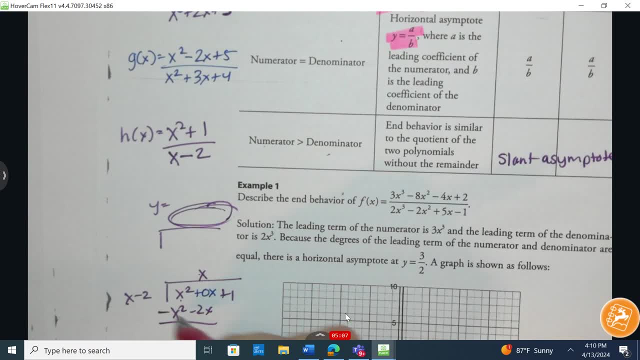 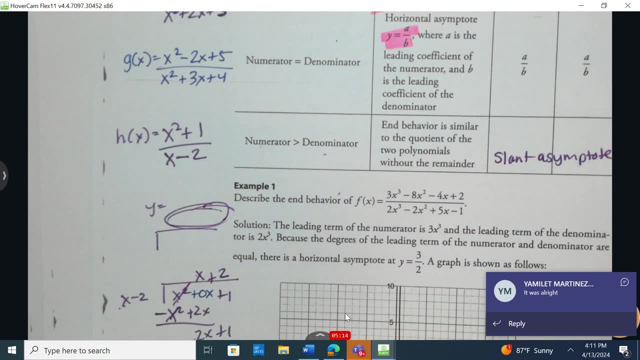 So I've got x squared minus 2x. Now I change the signs and I add straight down Additive inverses. bring down the one X times what equals 2x A two Multiply to get 2x minus four. 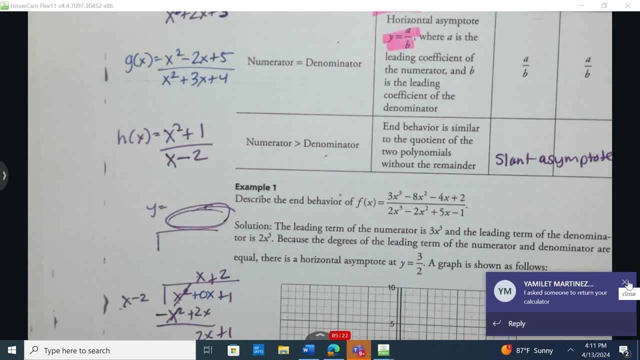 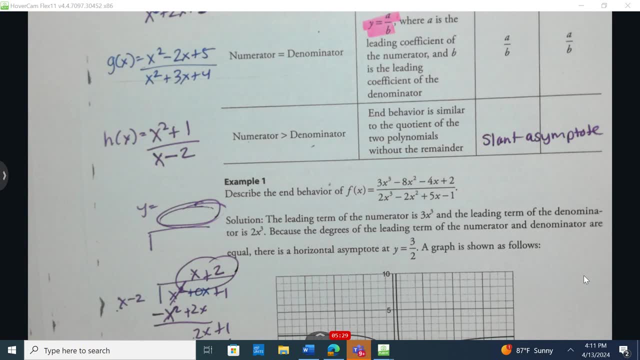 Change the signs, And what this says is: hey, we don't care about sorry. What this says is: hey, we don't care about the remainder. This is all we're going to be concerned with, So I'm going to press pause.